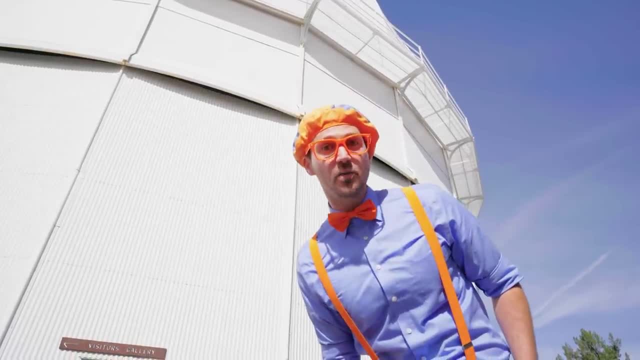 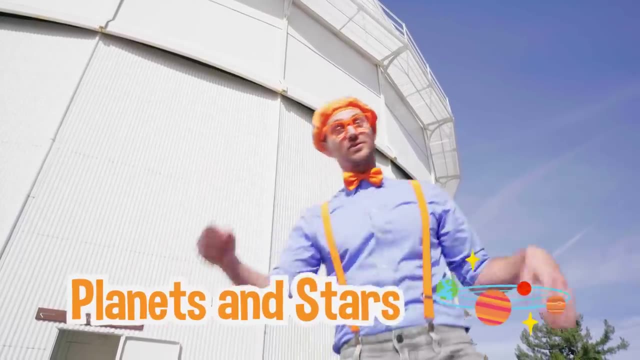 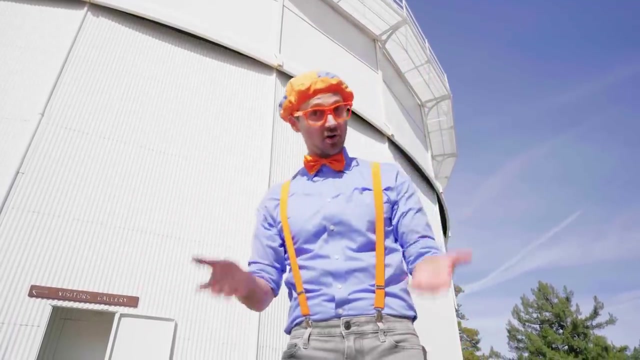 telescope inside there? Yeah, Do you know what a telescope is? Yeah, It's a piece of equipment used to peer out into outer space. You can see planets, You can see stars and all sorts of cool things. Yeah, The people that go into outer space are called. 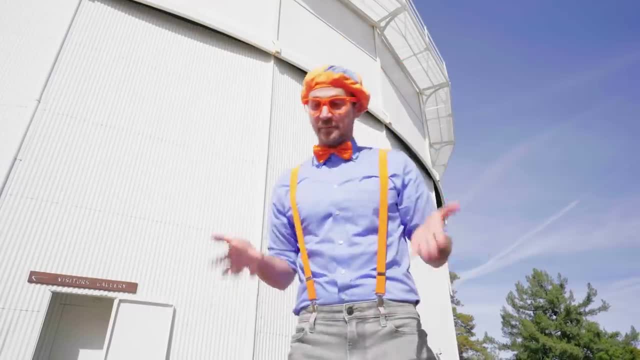 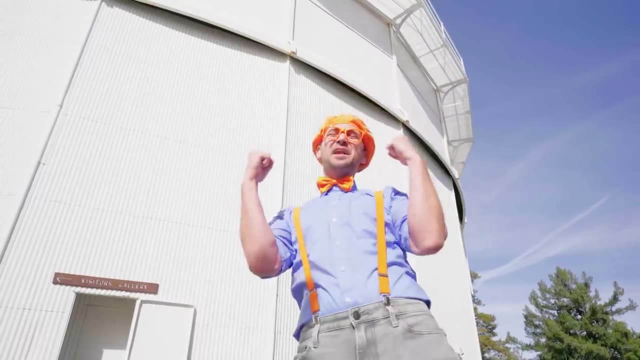 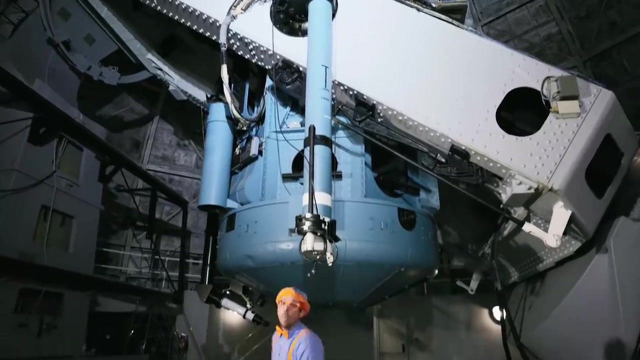 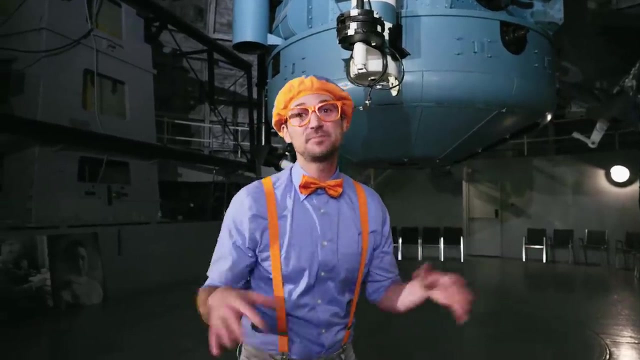 astronauts? Yeah, But the people from Earth that study outer space are called astronomers. Today, you and I can be astronomers. Let's go. Whoa, Did you hear that echo? Yeah, That's because we're in the dome, So cool. 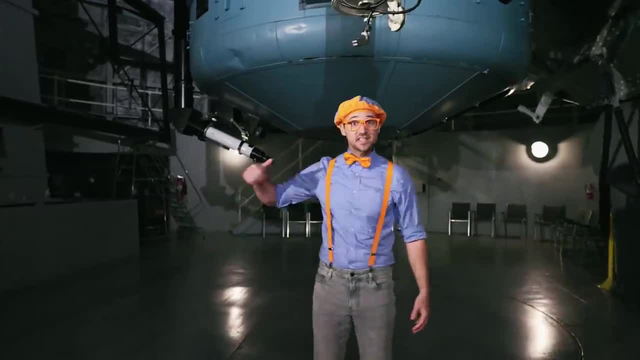 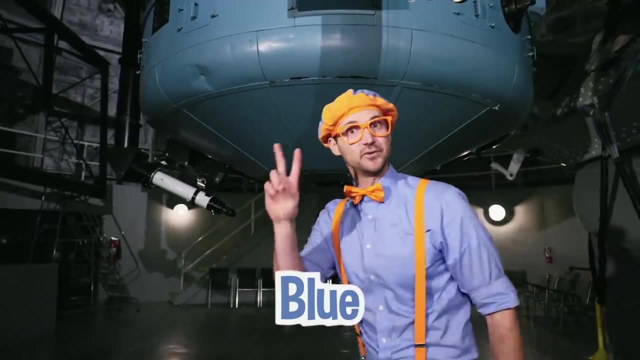 Yeah, And speaking of cool, yeah, Check it out. This is the telescope. Oh, I sure do love that color. Yeah, It's the color blue. You already know It's one of my two favorite colors, Whoa. 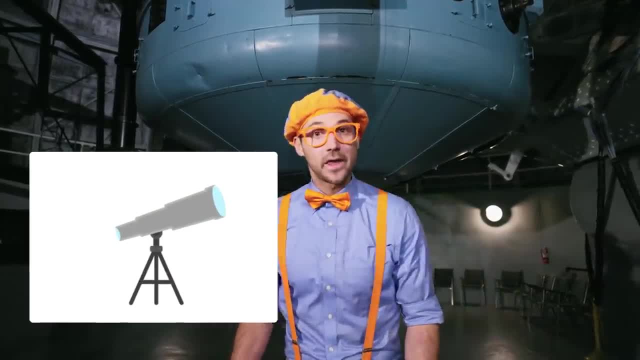 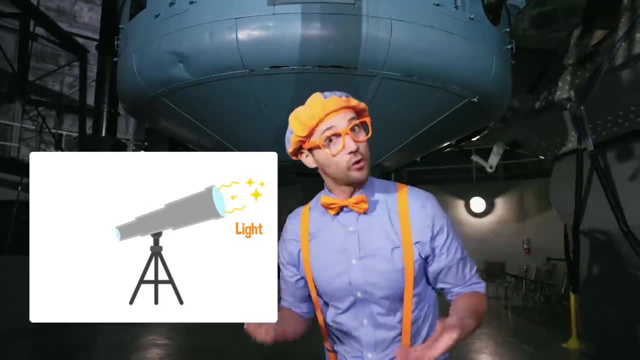 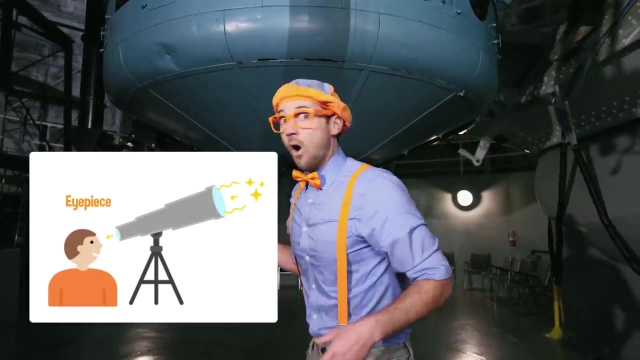 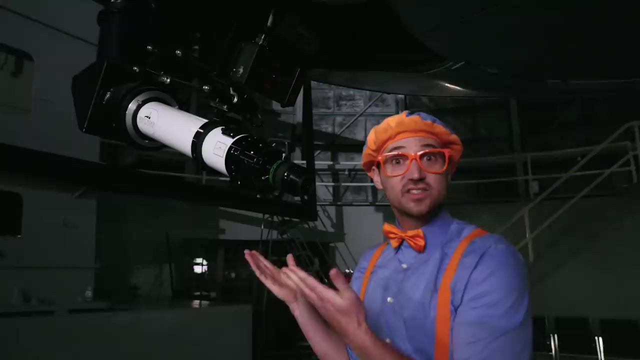 Do you know how a telescope works? Yeah, Basically, there's an opening up top way up there. Some light enters, say from a star or a planet, and then it bounces off some mirrors and then it goes to the eyepiece. The eyepiece, Yeah, Check it out. Yeah, This is what you look. 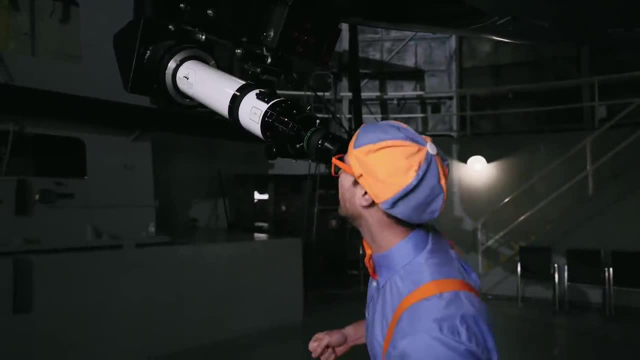 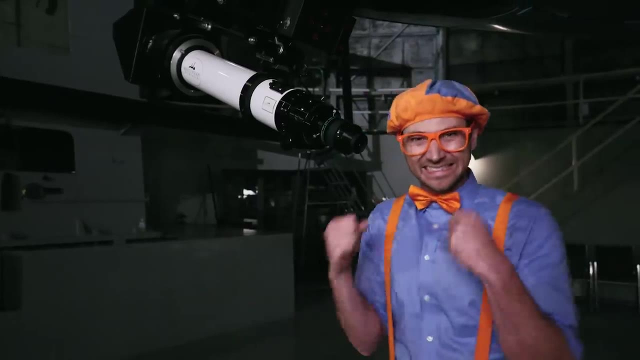 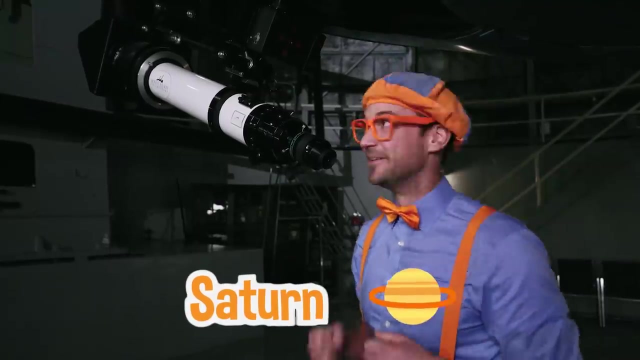 through to see things at night with the telescope? Whoa, Yeah, Do you want to see what you could see with this exact telescope if it was nighttime? Yeah, Whoa, Yeah. Do you see that That is the planet Saturn? Whoa, And I know it's Saturn because of all. 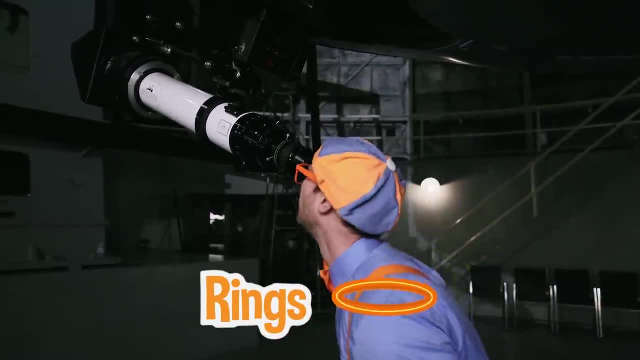 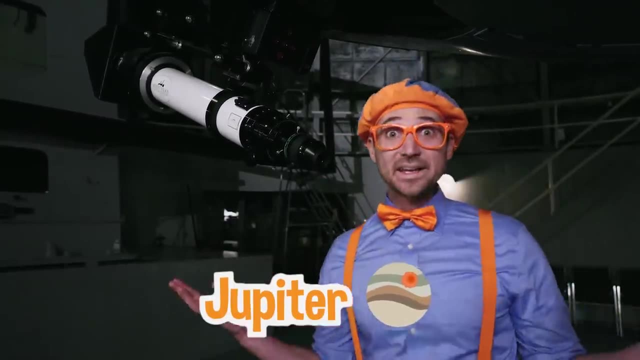 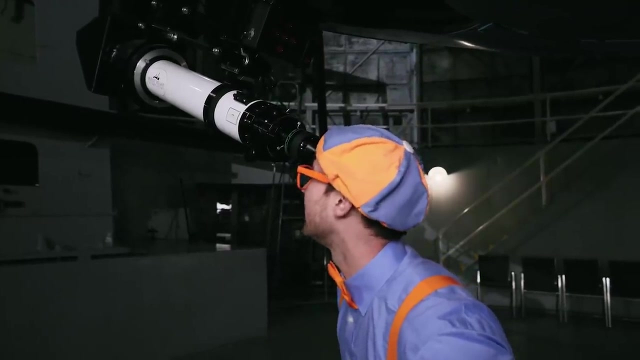 those colorful rings So cool. Whoa, And what's that? Yeah, That's our planet, Jupiter. That's the biggest planet in our solar system. Whoa, It's so big. Whoa, And it looks like Jupiter has a lot. 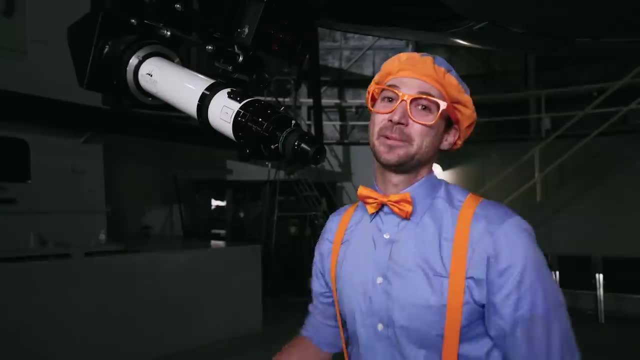 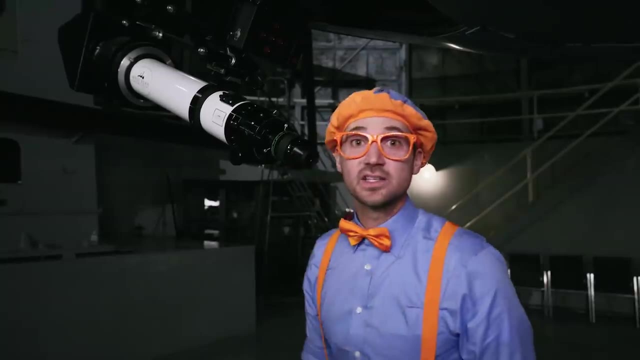 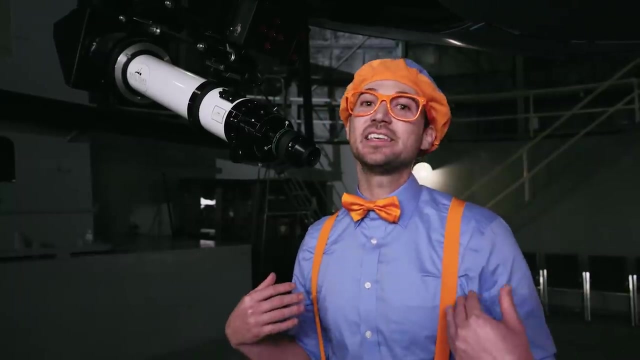 of moons. Wow, Yeah, Planet Earth, we only have one moon. Whoa, Whoa. look at that. Yeah, Looks like Andromeda Galaxy. That is the closest galaxy to our galaxy. Our galaxy is the Milky Way Galaxy- Whoa. 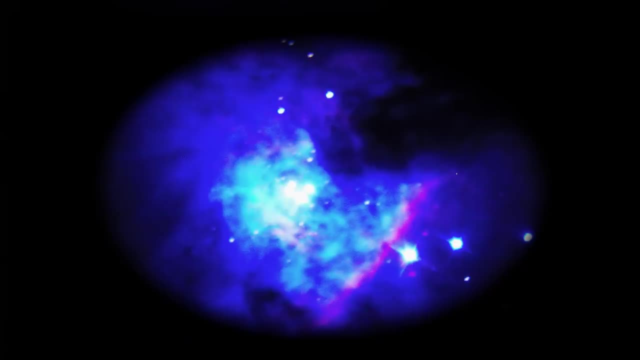 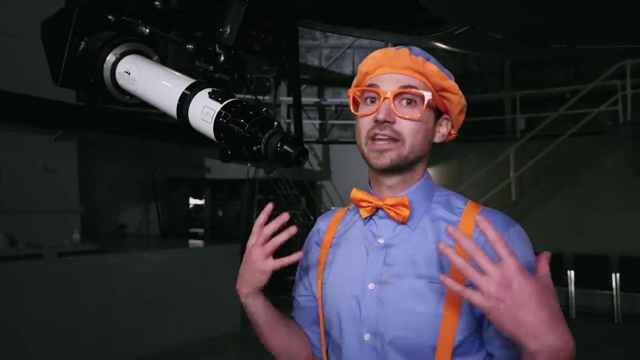 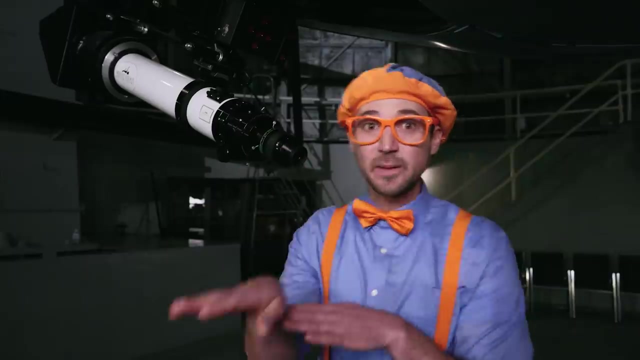 Whoa, And what's that? Ooh, Orion Nebula- Yeah, That is where all the stars are born in our galaxy galaxy. Whoa, This telescope is awesome And how it sees all these things in outer space. since they're in different locations, that means this telescope moves. 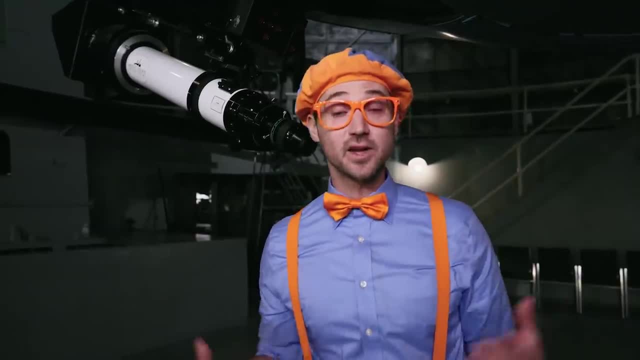 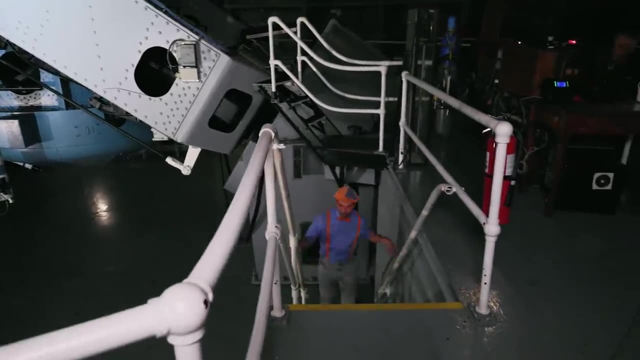 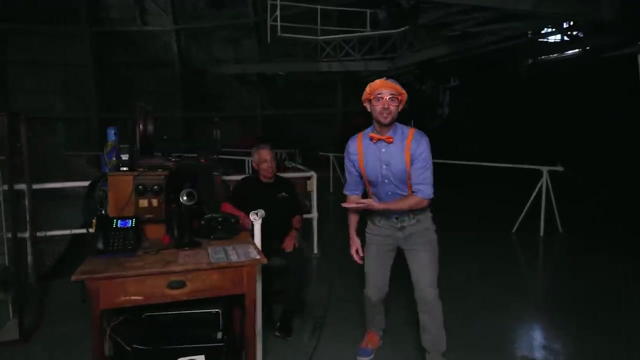 Maybe we can go to the control board and move the telescope ourselves. Yeah, let's go. Whoa, So many stairs. Whoa, Oh, who are you? Hi, I'm Tom. Oh, nice to meet you, Tom. I'm Blippi. What do you do here? 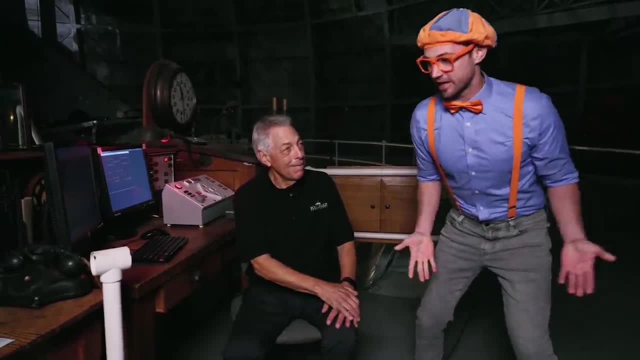 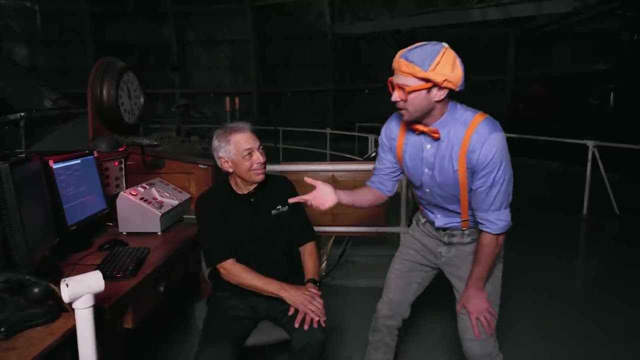 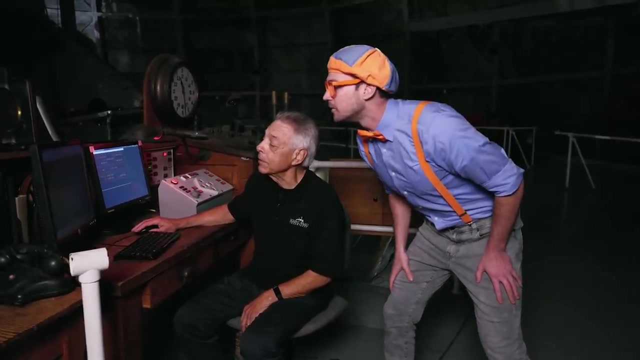 I'm the telescope operator. Oh, the telescope operator. So that means you push buttons to make the telescope go left, right, up down. That's right, Wow, Why do you have a computer here, Tom? This tells me the address of what I want to look at, If I want to look at this star. 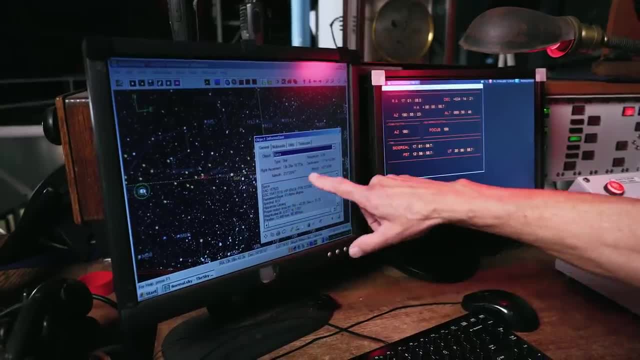 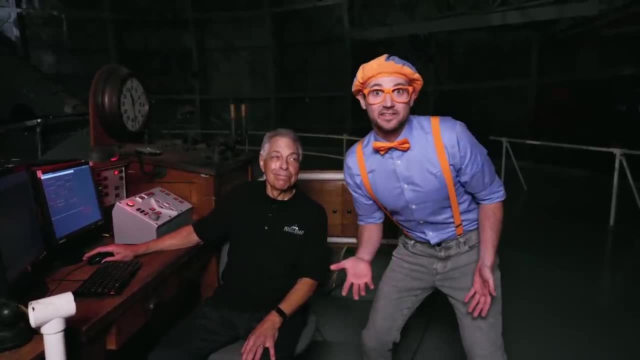 it tells me where to look. Wow, That's really cool. He needs a computer to have the address of, say, a planet or a star, and that tells him where to point the telescope at. Oh, that is really cool. Why do you have a clock way over? 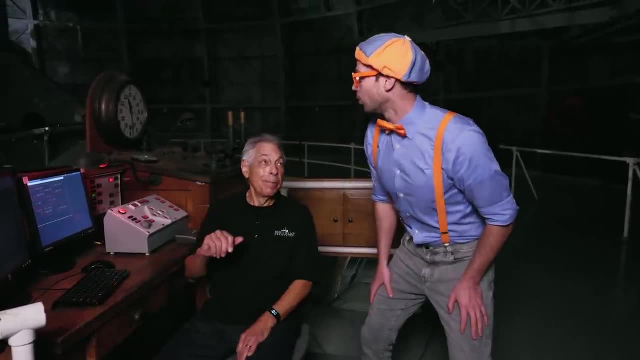 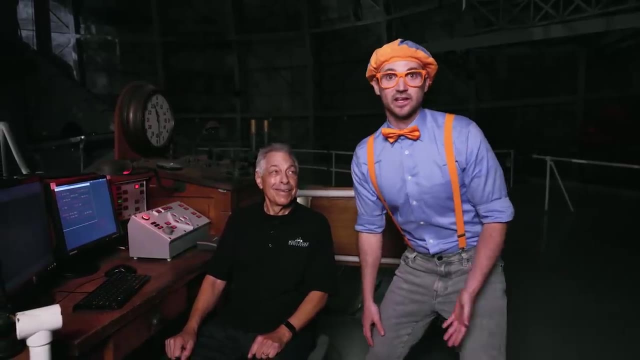 there. Well, I have to tell the time. This is star time. Oh, star time. Exactly, It's called a sidereal clock. Oh, a sidereal clock. Oh, that makes sense. Yeah, you can't look at stars during. 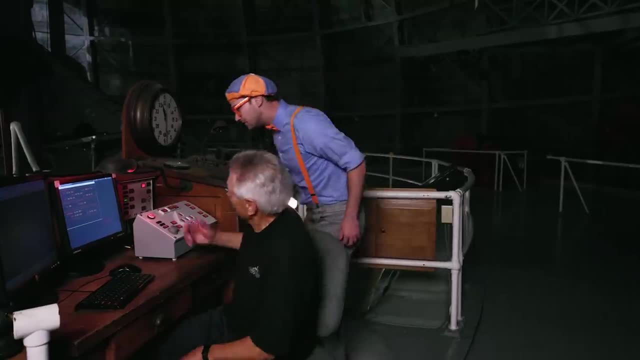 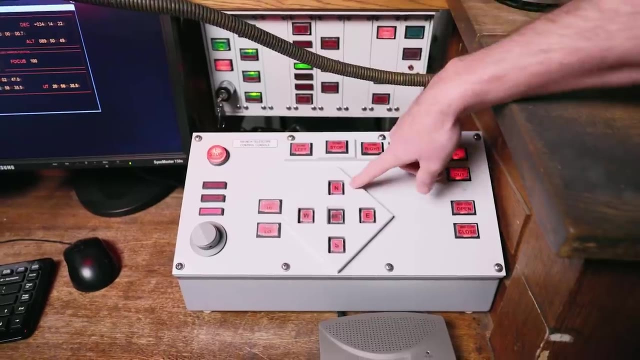 the day. Oh, and what are all these buttons? These are to move the telescope I have to point, move the scope To the star or object I want to look at. Ooh, N-E-S-W, North east, south, west. 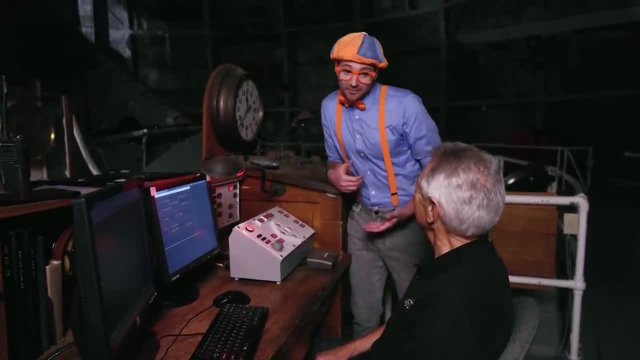 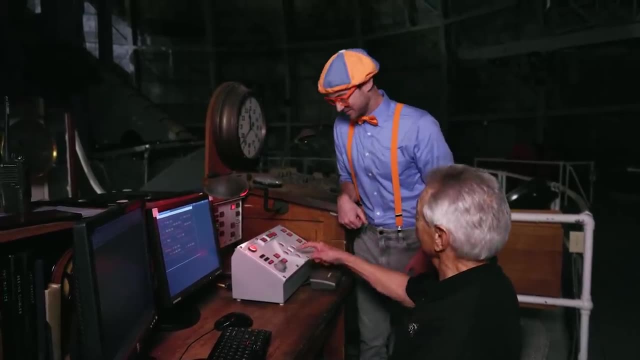 That's right. Oh, cool, And Tom, do you mind if we like, operate the telescope and maybe make something move? Sure, Let's open up the dome first. Cool, Would you push that button please, This button? Yes, All right, here we go. 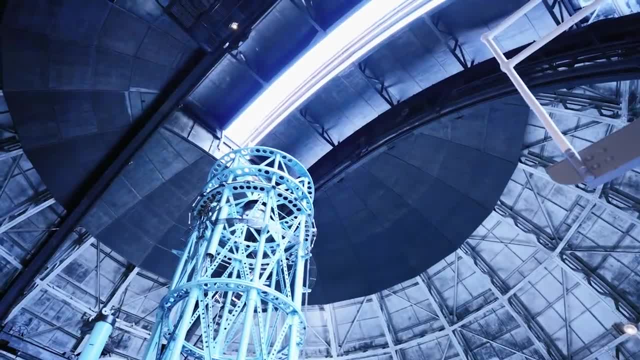 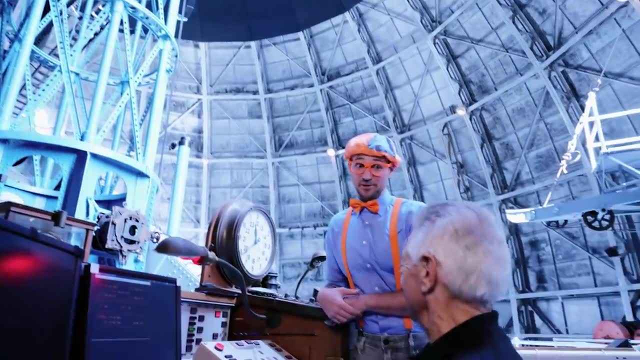 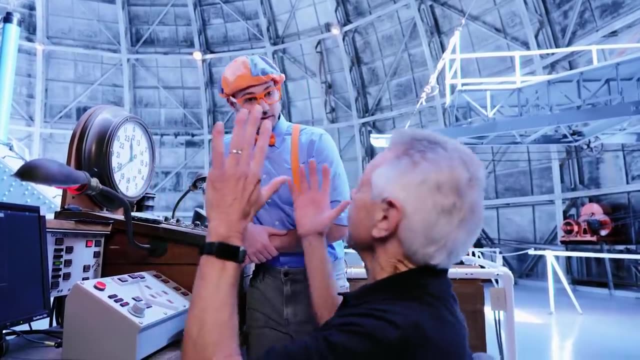 Whoa, What do you think? That was really cool. Thanks for letting me do that. And what else does the telescope do? Well, we have to move the dome around, We have to point it in different directions. Wait here a second, Let me. let me show you. Okay. 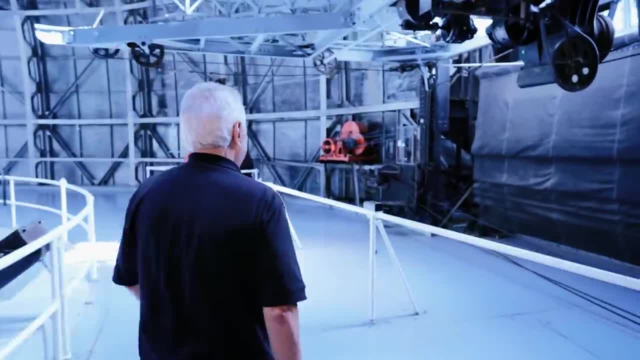 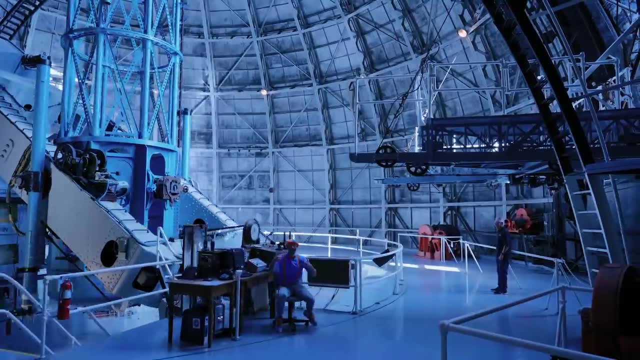 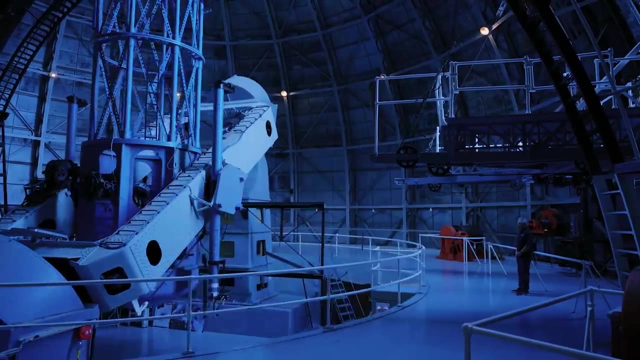 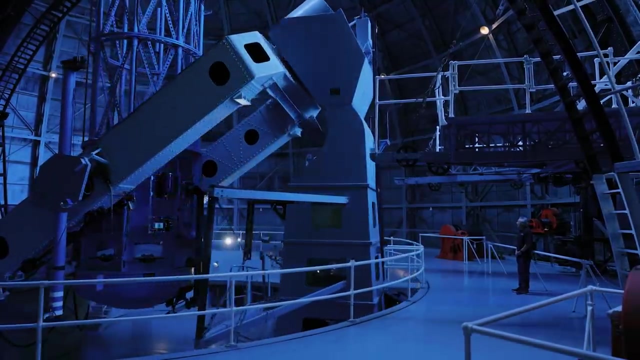 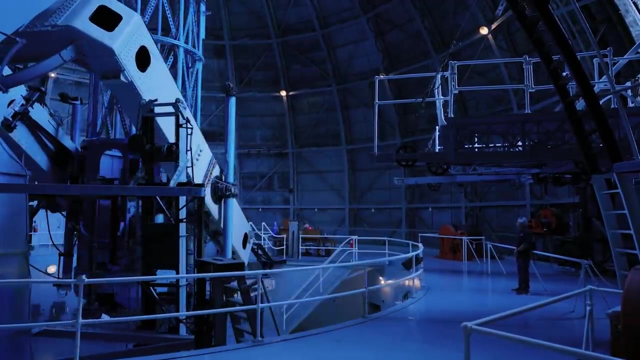 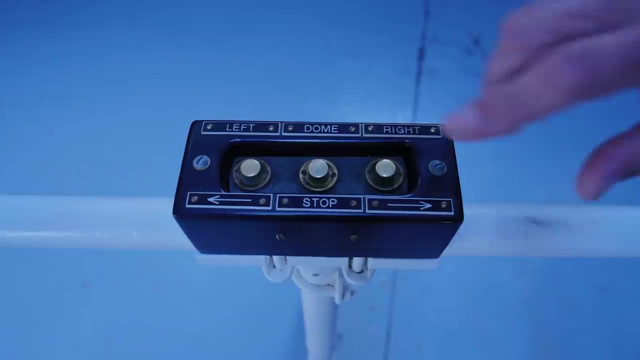 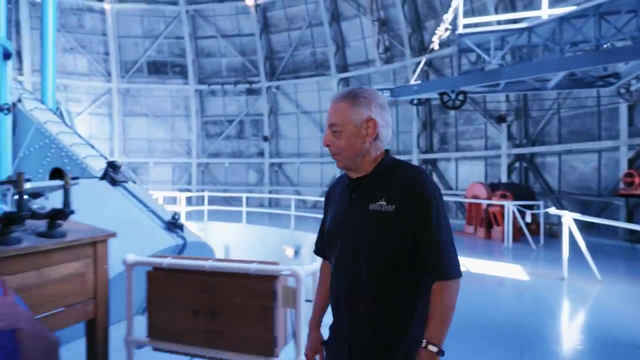 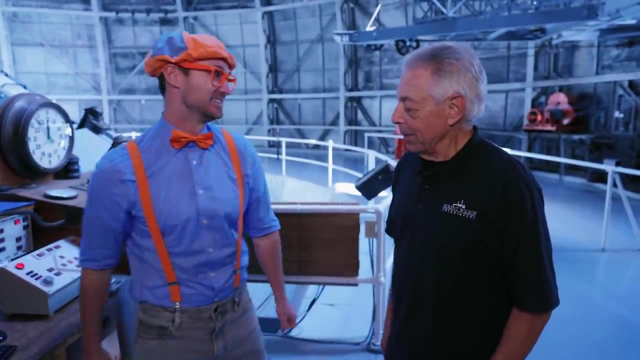 Are you ready? Yes, Here it is. what do you think of that? wow, that was awesome. thank you so much for showing me this awesome telescope. glad to have you here. all right, see you later. so long bye-bye. 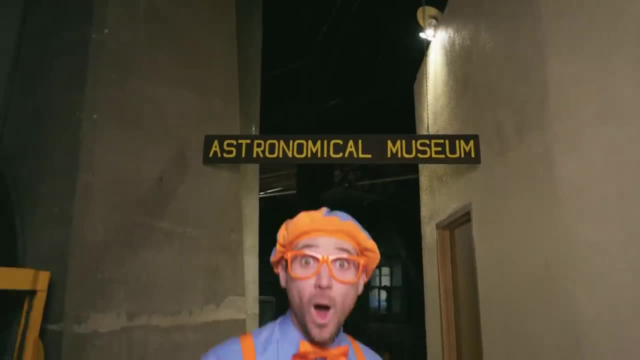 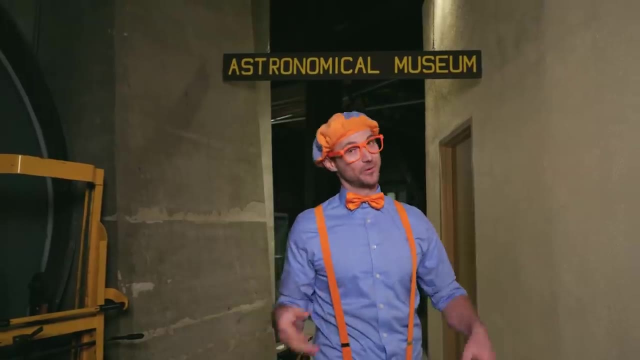 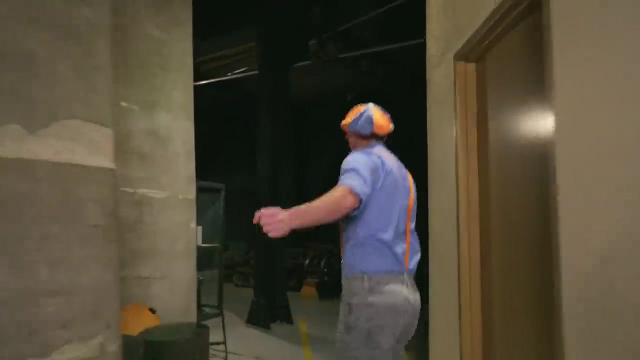 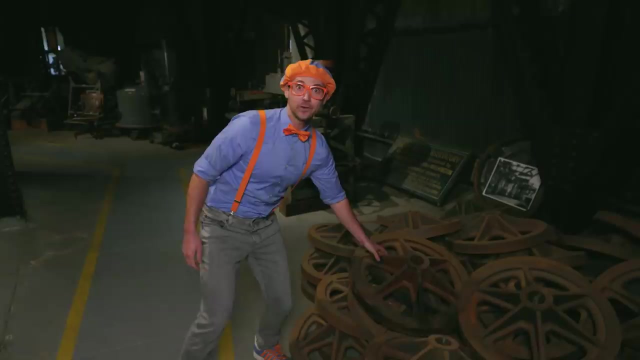 hello, check it out. we're at the astronomical museum, yeah, and at this place they have a lot of really cool old gadgets that they used to use to learn about outer space. shall we look at these? whoa, they look like wheels, yeah, like wheels on the car, but actually 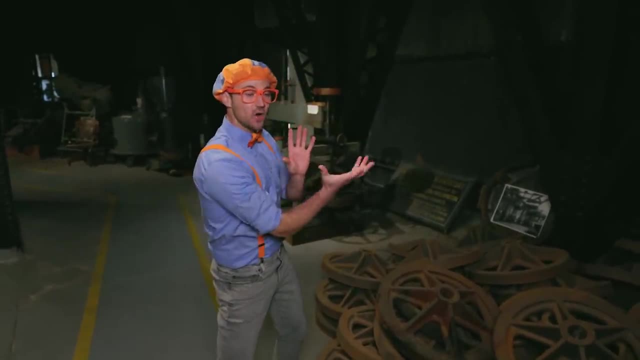 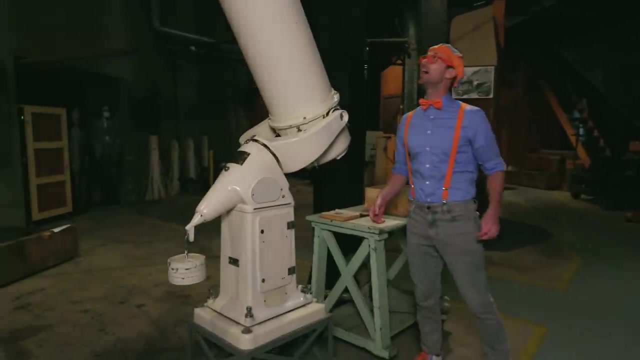 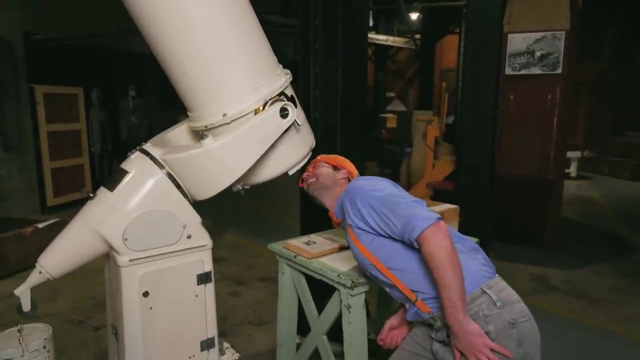 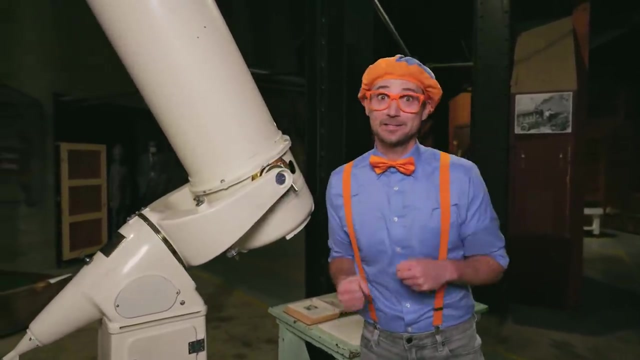 these are wheels that are on the dome, so then the dome can spin around. so cool, whoa. yeah, i know what this is. it kind of looks like a telescope, doesn't it? yeah, oh, yeah, oh, you can see stars with this, planets, whoa, other galaxies maybe. oh cool, excuse me, 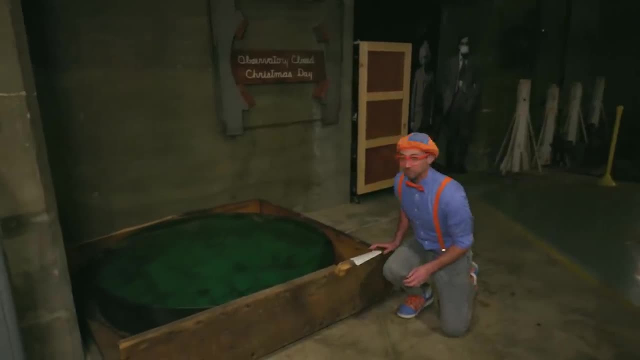 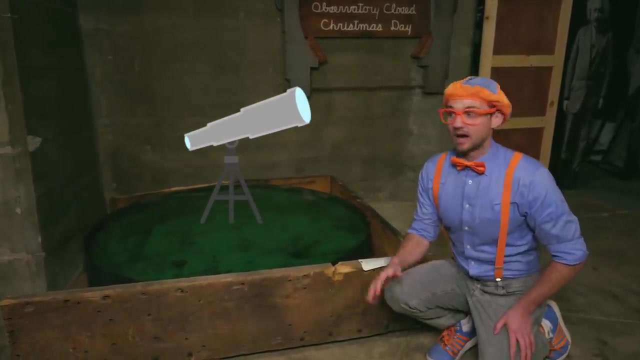 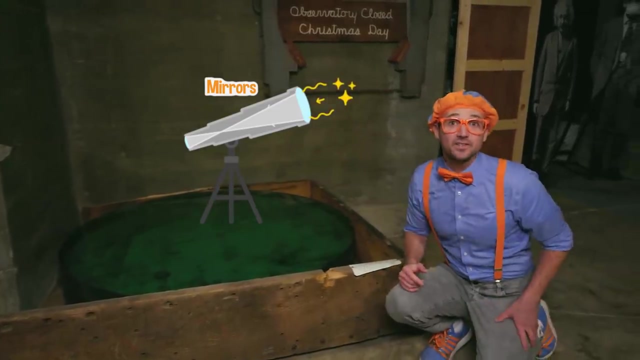 whoa, look, this is a really big piece of glass. wow, yeah, remember how telescopes work. yeah, oh yeah, you have a mirror and another mirror and light bounces back and then eventually, after it bounces off a couple mirrors, then it goes into the eyepiece and this piece of glass used to have. 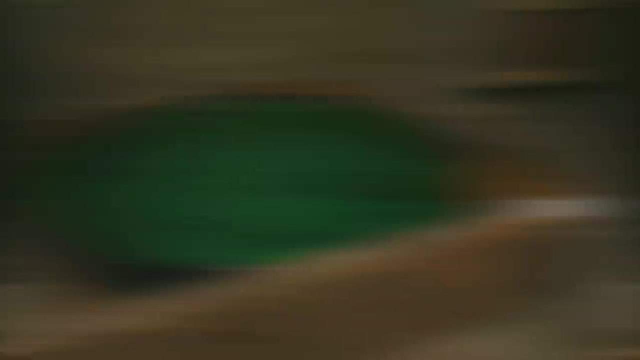 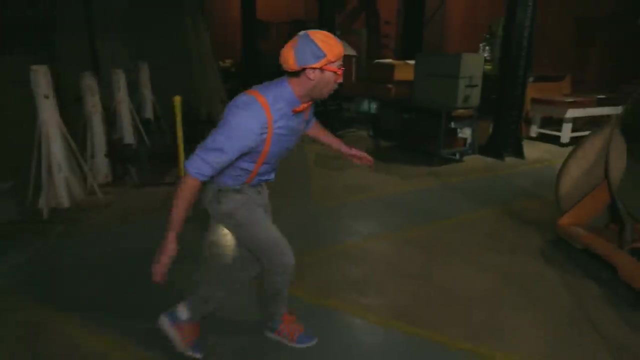 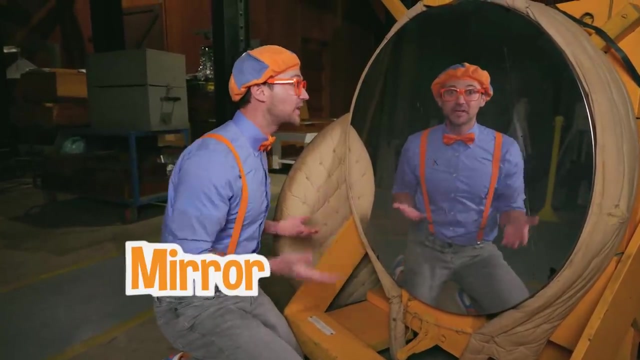 silver on it. so then it was really shiny like a mirror. oh, speaking of mirrors, look, there's a mirror right over there. whoa, oh hello. yeah, this mirror came from a real telescope, a very, A very old one, of course. Yeah, because we're at a museum. 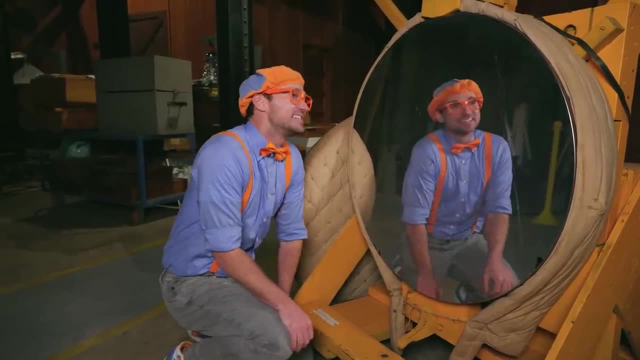 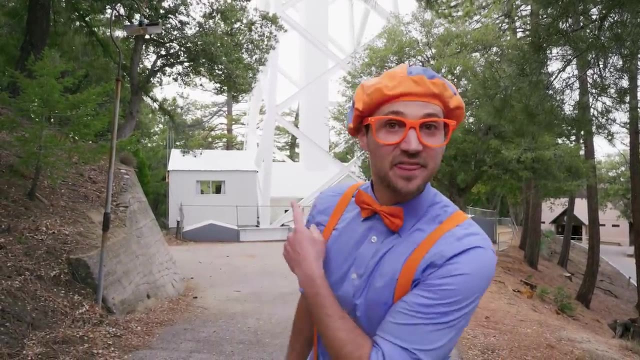 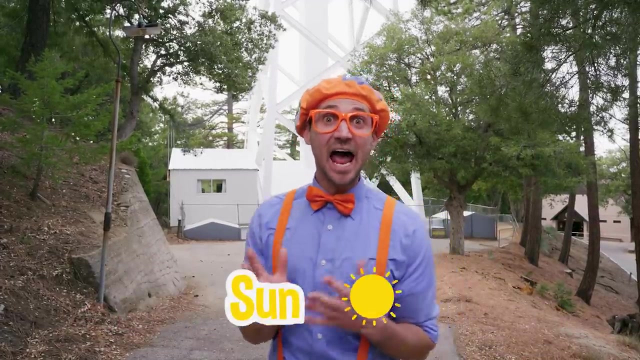 Well, shall we keep learning about telescopes and outer space? Yeah, Whoa, check it out. Another telescope, And this is the 150-foot solar telescope. Solar means sun. Yeah, this telescope, you can look at the sun. 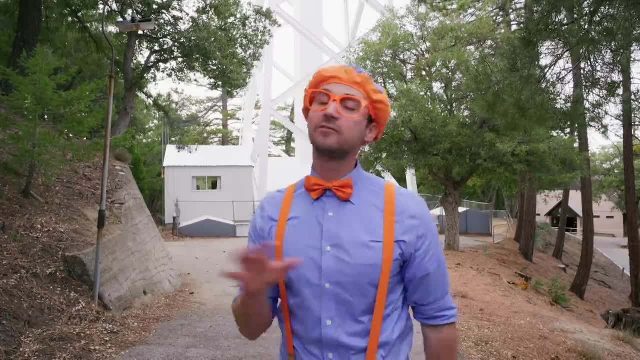 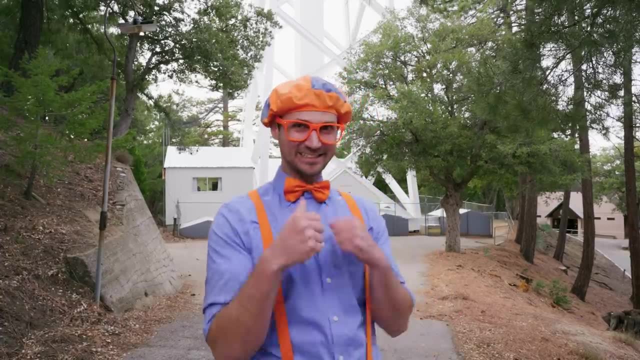 Okay, before we go in, I have to tell you: never look at the sun unless you have a solar telescope. Okay, it's very important. It's not good for our eyes. Good job, All right, let's go Wow. 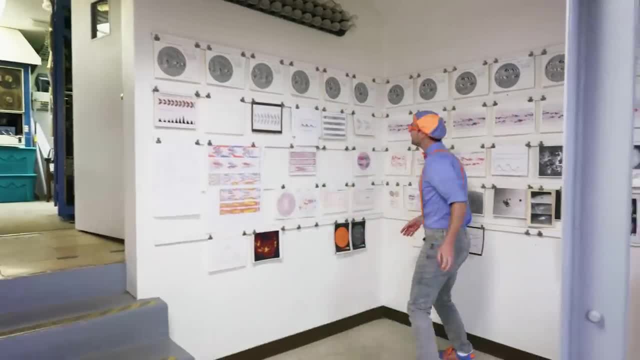 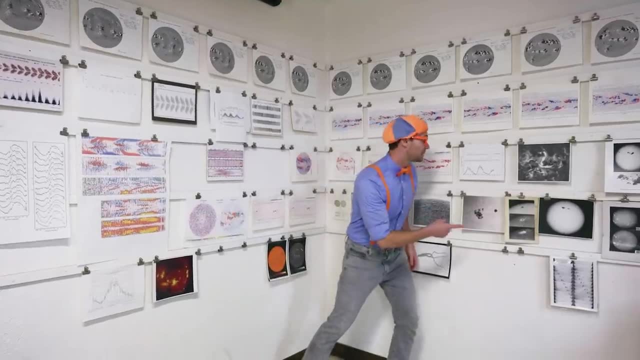 Whoa cool, check this out. Whoa, look at all of these charts- Whoa. and graphs. Ooh, and some pictures of the sun. Yeah, we're definitely in the right place. We're in the right place to find the solar telescope. 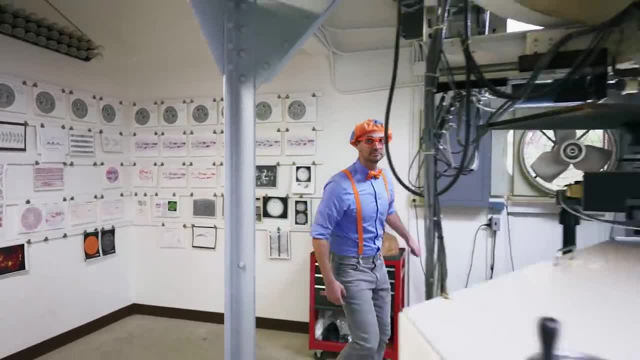 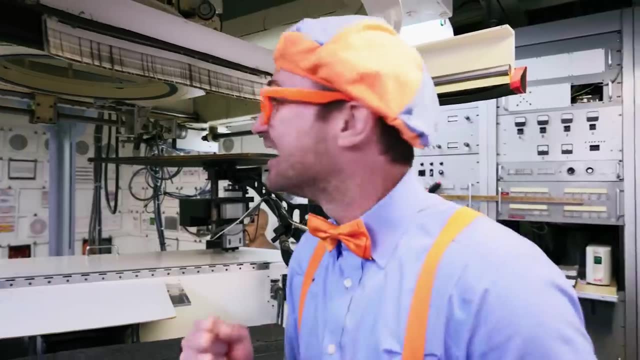 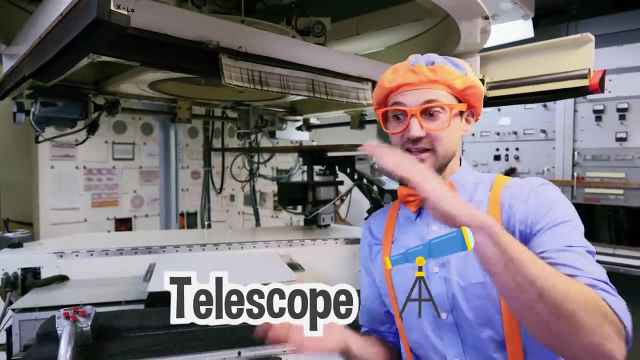 Let's see where could it be. Hmm, whoa cool here it is. It is so cool. And remember how I said: it's a 150-foot solar telescope? Yeah, that's because the telescope itself is 150 feet tall. 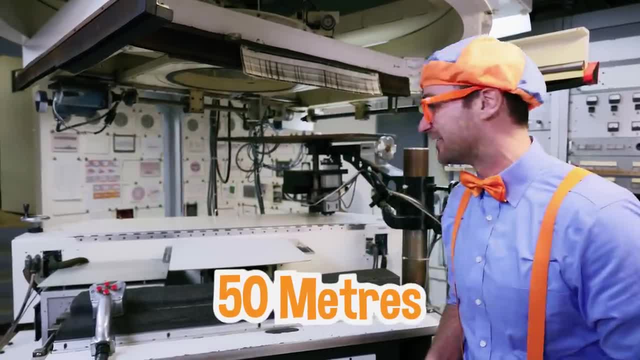 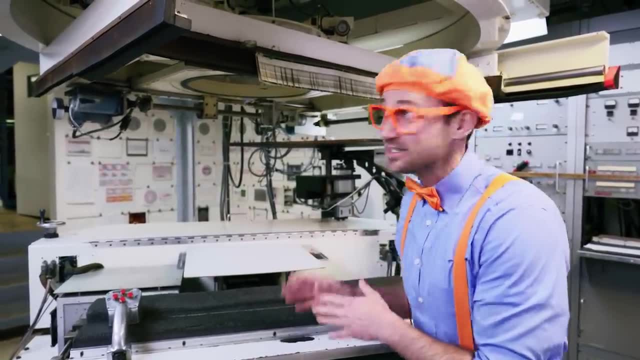 Yeah, that's really tall. That's about 50 meters. whoa, All right, you never want to look directly at the sun, okay, And the only reason why we're going to be able to see the sun is because we're using a solar telescope. 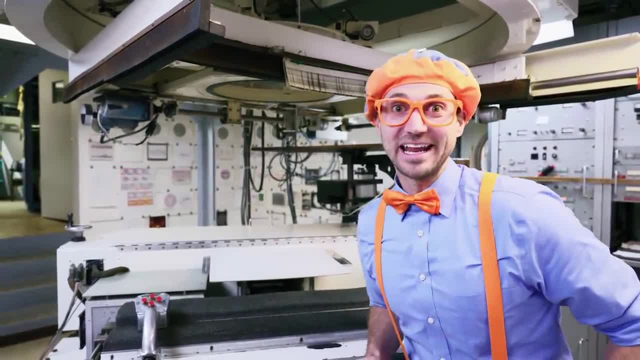 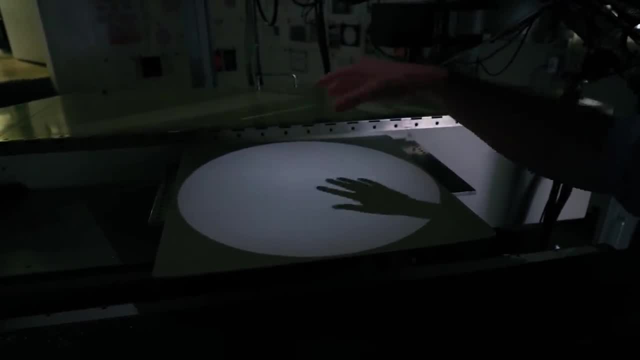 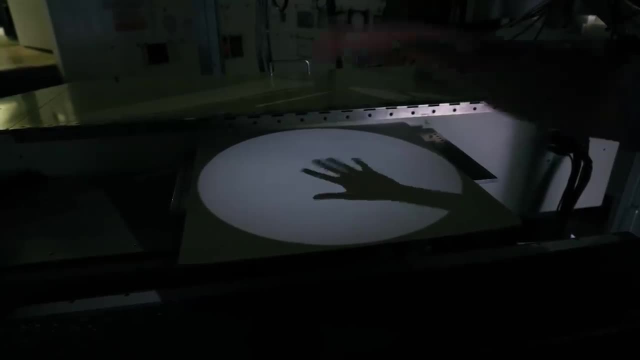 not a normal telescope, a solar telescope. All right, are you ready? Ha-ha, Oh, whoa, check it out. Whoa, do you see this? Yeah, this is a live image of our sun. yeah, This light is coming down and hitting. 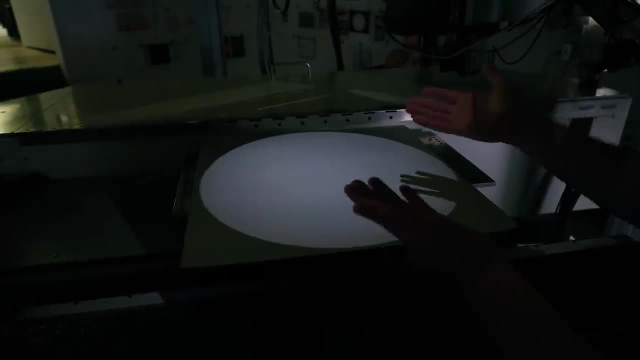 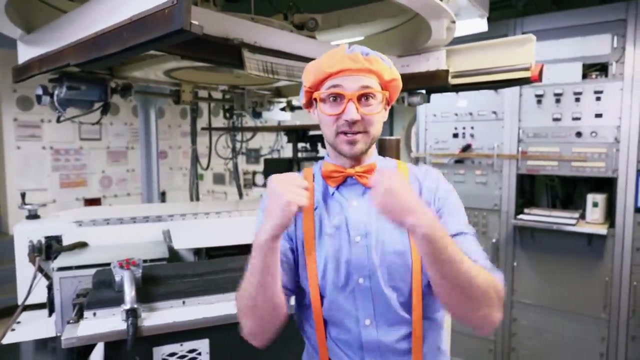 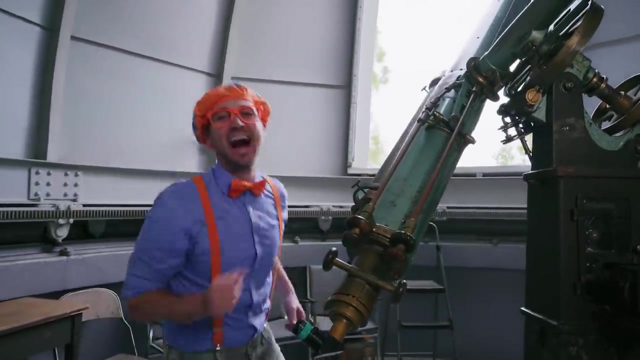 this white piece of paper? yeah, so we can see our sun right now. This is so cool. Whoa, I love solar telescopes. yeah, Whoa, I think we're in outer space. Five, four, three, two, one blast off. 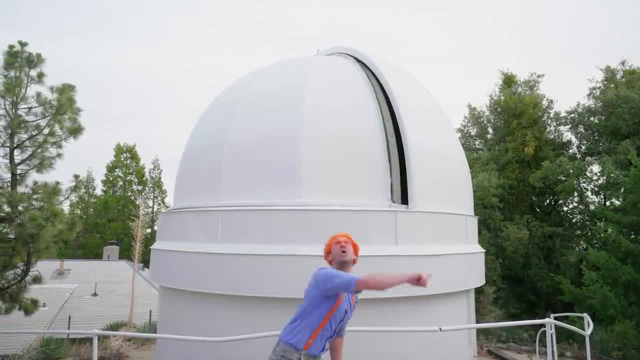 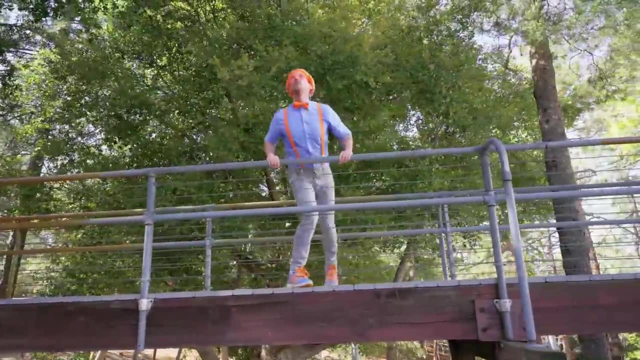 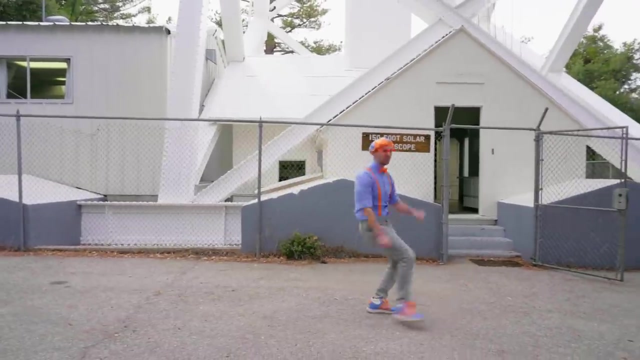 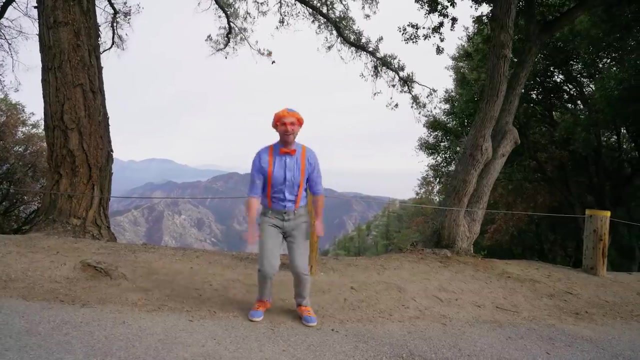 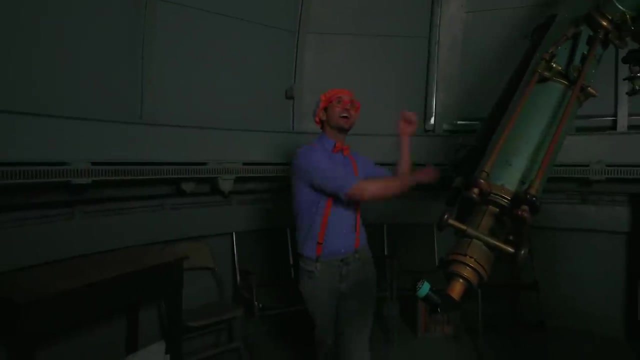 Blast off thousands of miles an hour Using all of that big rocket power. It's so loud, oh, you just can't ignore it. See you later as we fly out of orbit. I'm a rocket that can take you into outer space. 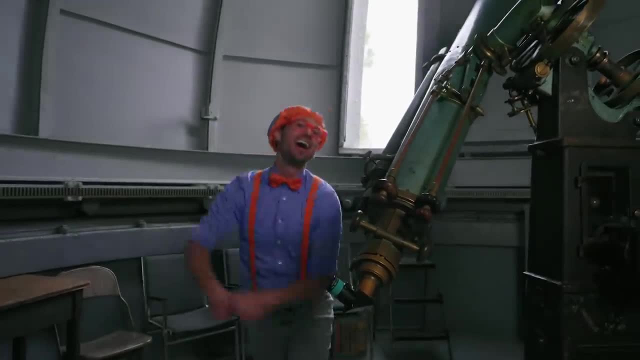 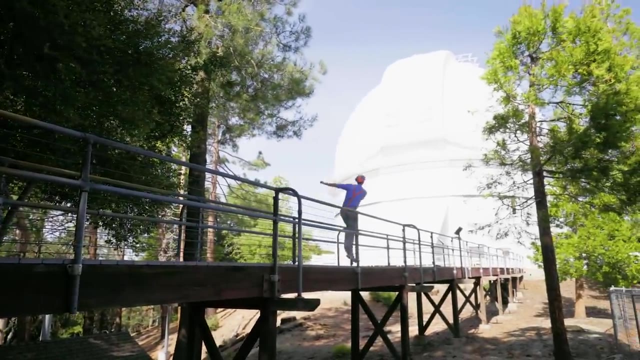 Maybe you and aliens will come face to face. I'll take you on a journey to the stars and back, making our own space. We ain't going away because we ain't got no track and so we need to use a seatbelt. 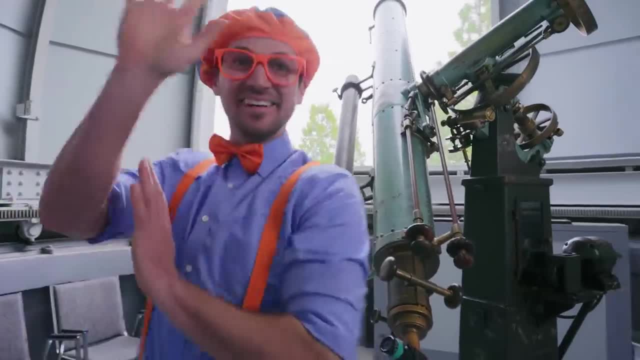 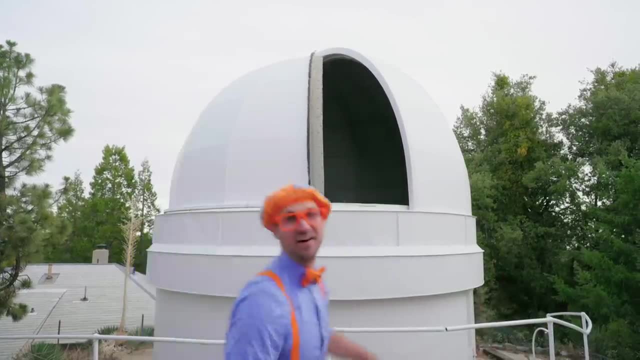 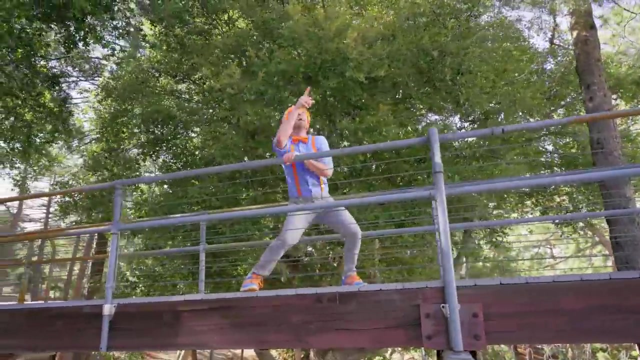 There's no gravity. We are searching for something planetary Heading home for Earth. We do it gradually. Got to get back home to humanity. Blast off thousands of miles an hour Using all of that big rocket power. Blast off thousands of miles an hour. 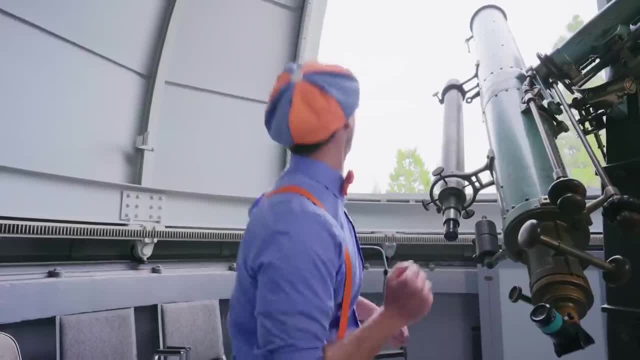 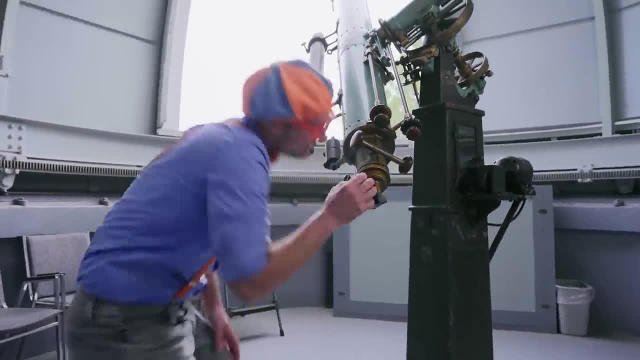 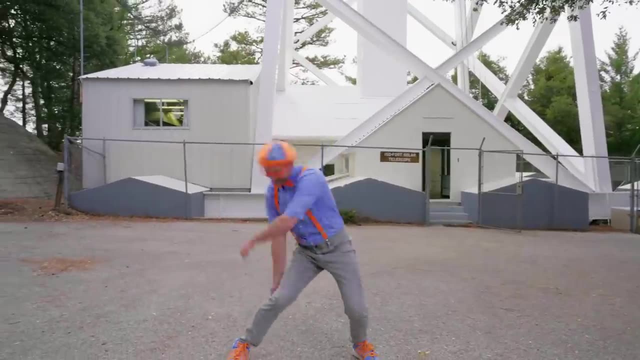 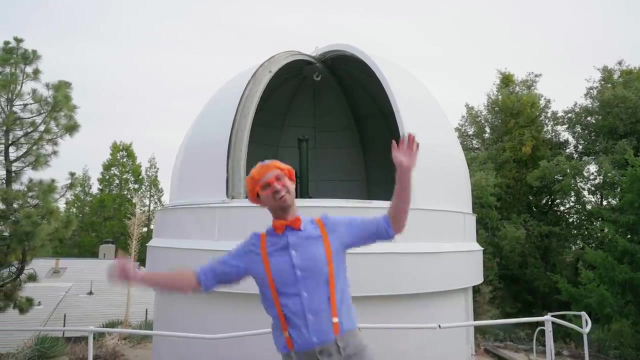 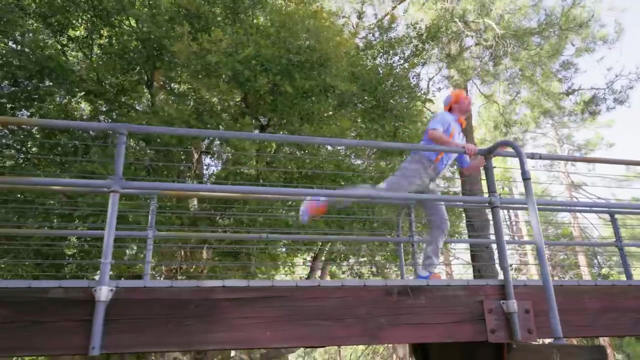 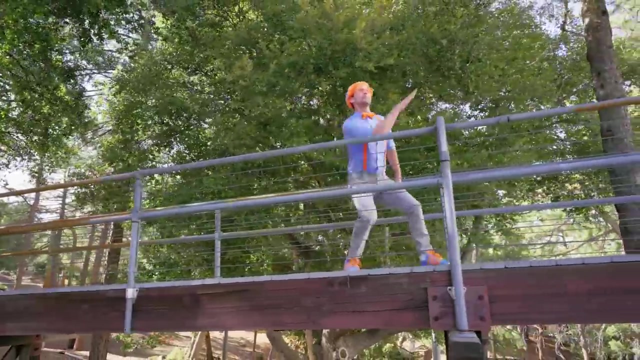 It's so loud. oh, you just can't ignore it. See you later as we fly out of orbit. Fly my rocket far away, Flying far away in outer space, Blast off from the base, Taking off to outer space. Fly my rocket far away. 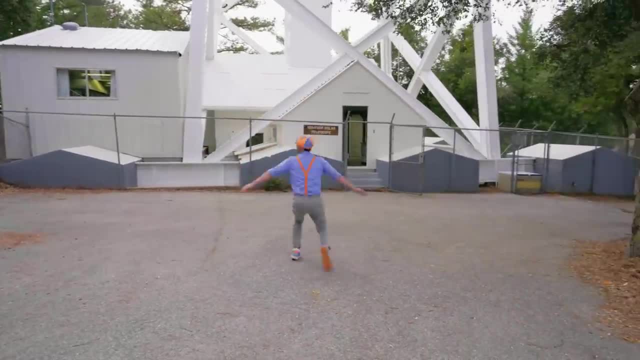 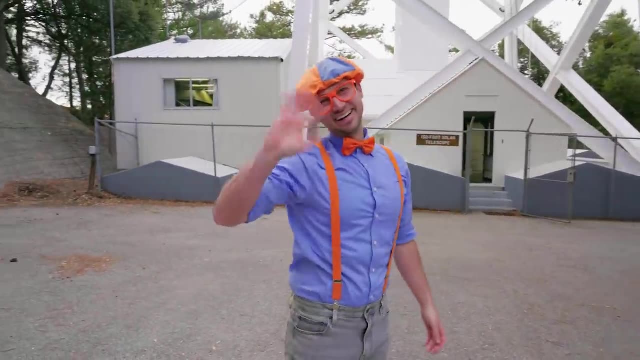 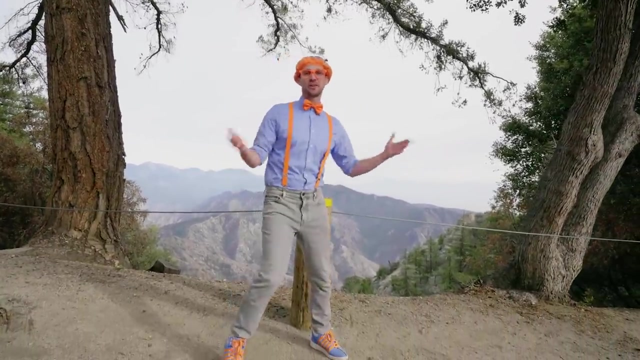 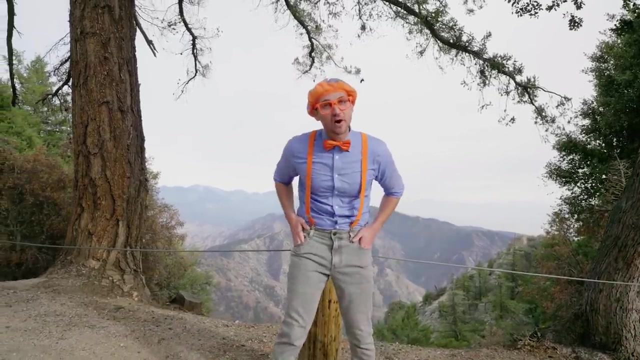 Flying far away in outer space, Blast off from the base, Taking off to outer space, Woo-hoo-hoo-hoo. Hasn't this been so much fun: learning about outer space and telescopes together. Yeah, Hey, do you know how many planets are in our solar system?